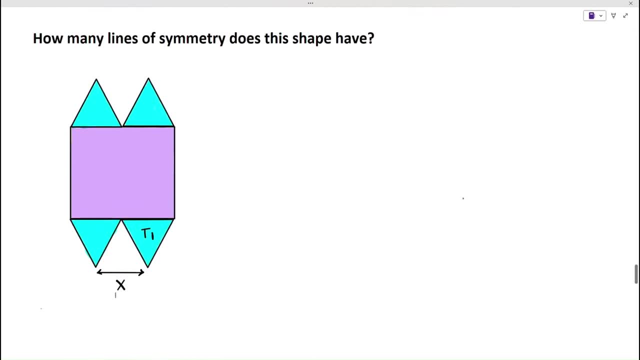 How many lines of symmetry does this shape have? So we know that with lines of symmetry that on either side of the line the shape must look the same. So let's draw the lines of symmetry we can find. So one line of symmetry we can find is vertically down through the middle of the shape. 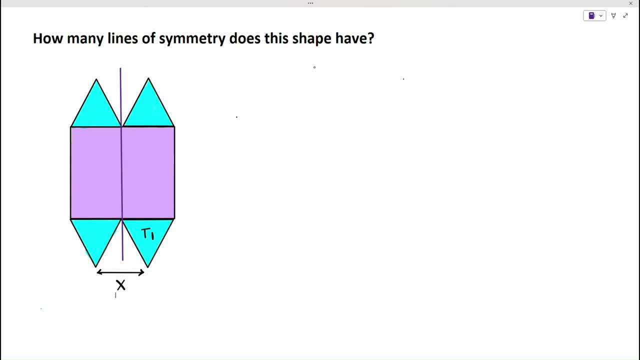 And another line of symmetry we can find is horizontally across the middle of the shape. Now you can't find any more lines of symmetry, And so this shape has two lines of symmetry. Now let's approach the third part, Our question: What is length x? 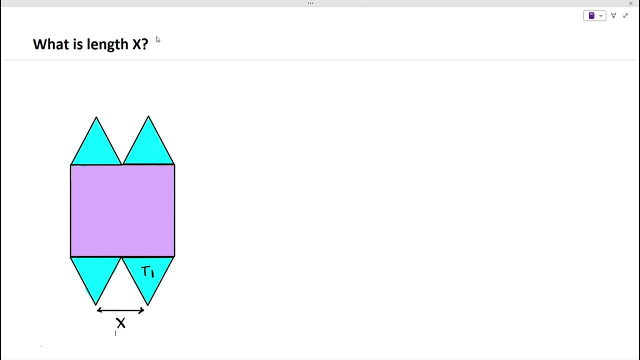 So we're told in the information that we were given at the beginning that all the triangles are equilateral triangles. So we can draw a line between the two top corners of the triangles at the bottom And we can make another triangle between them. We can highlight that triangle. 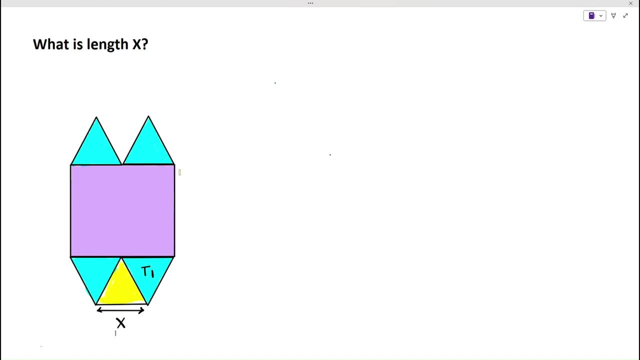 And this triangle is the same as the other ones as well. So this is also one of those equilateral triangles, And you can see in the diagram that two equilateral triangles share one side of the square. So in the first part of our question we found out that the length of one side is 42 centimetres. 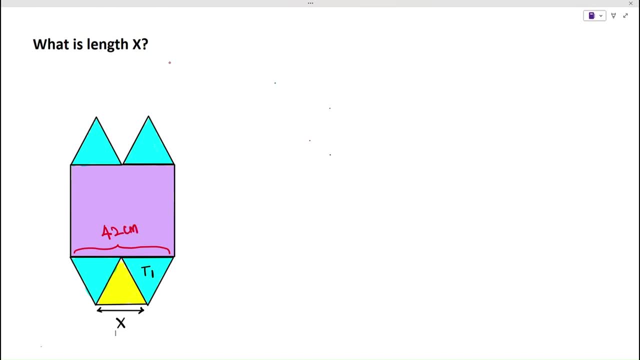 Since the two triangles share one side, we do 42 divided by 2 to get the length of one side of our triangles, And this is a nice simple division. This is 21 centimetres, And so with an equilateral triangle, we know that all three sides have the same length. 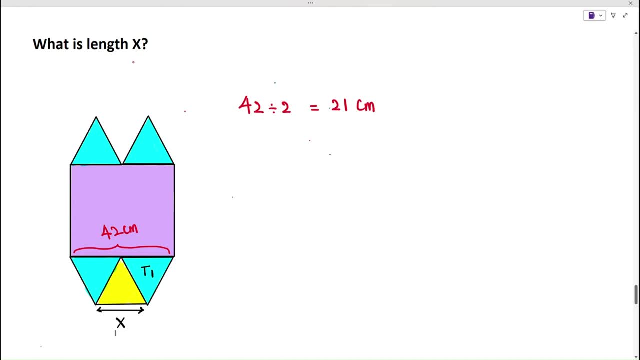 And since the triangle that we have drawn additionally has the same length as the other triangles, length x will also be 21 centimetres. Now we'll approach the fourth part of our question. What is the area of the square? So we've been told. 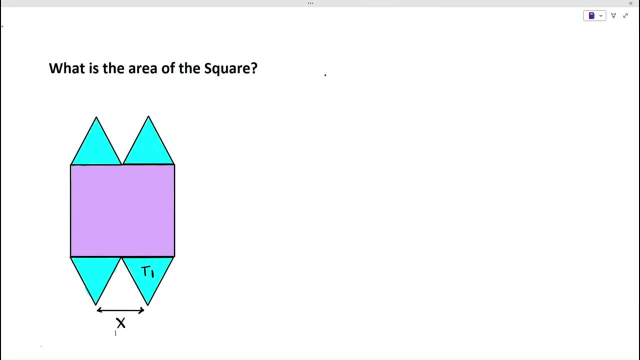 Well, we found out, actually, that the length Of one of the sides of the square Is 42 centimetres, And so, to find the area of the square, multiply the base By the height, Or the length by the width. 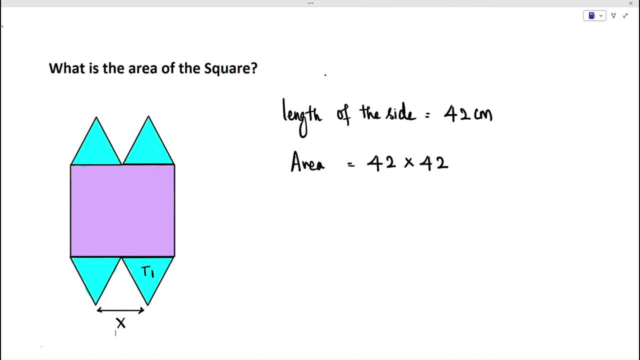 And so we get 42 times 42. And so What we're going to do first Is we're going to multiply our 2 to 2. So we get 4.. And multiply 2 with our 40. So we get 8.. 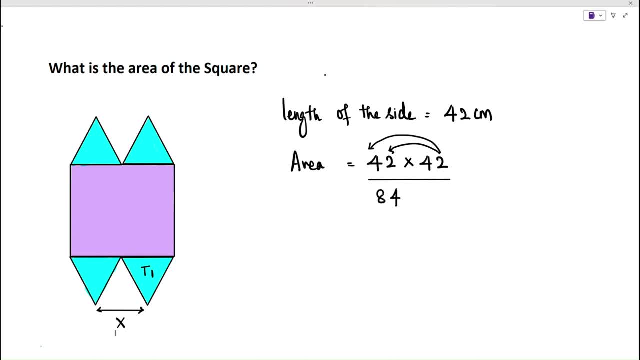 In our tens column. So we get 84. Now we add a 0, because we're going to multiply by 40 this time. So we have 4 times 2, which gives us our 8. And 4 times 4.. 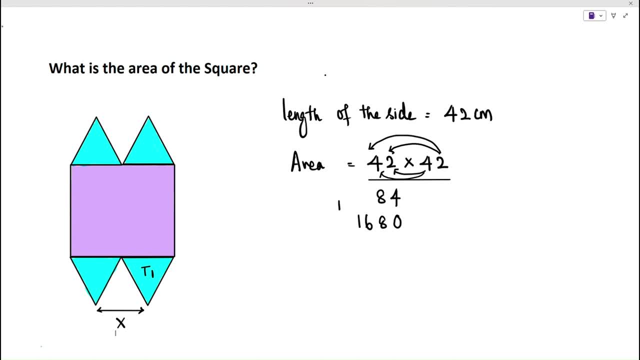 Which gives us 16. This gives us 1,600.. And 80. And so if we add the two values of 84 and 1680 together, We get 40 is 4.. 8 times 8 is 16.. 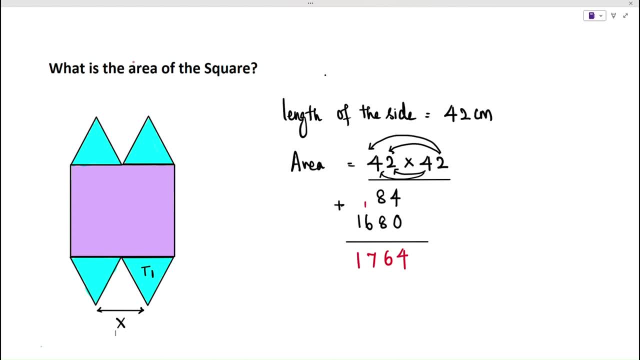 We carry the 1 over. 1 plus 6 is 7. And we have our 1 here. So the area of our square Is 1,600.. 1,764. Centimetres squared. Now we approach the final part of our question. 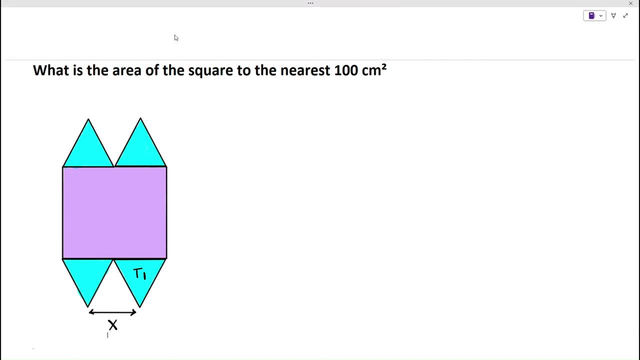 What is the area of the square To the nearest? 100. Centimetres squared. So we have the area As 1,000.. 764. Centimetres squared. Now Let's draw a number line. So.